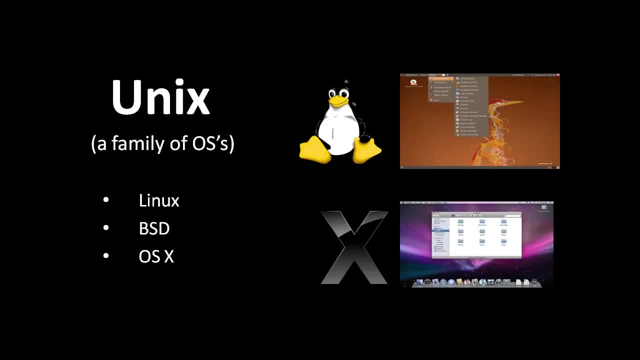 that are free and open source and developed by Microsoft. The Unix OS is developed by a scattered community around the world. Apple's OS X was originally based on a variant of BSD, but is itself proprietary and only legally available for Apple's own computers, even though the underlying Apple hardware is the same as standard PC hardware. 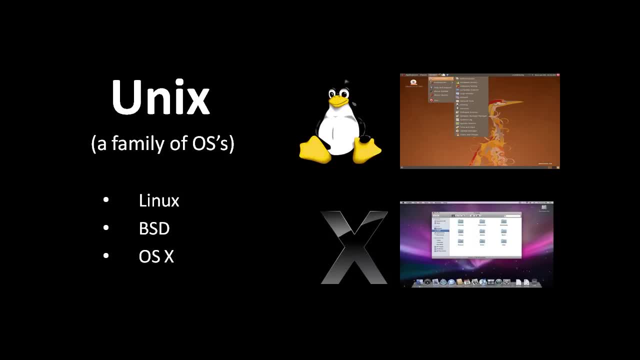 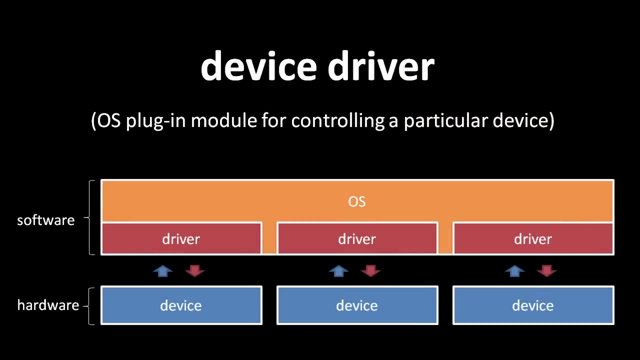 Except when we discuss file systems, all of the information in this unit will be platform agnostic, applicable to both Windows and Unix systems. A device driver is a plug-in module of the OS that handles the management of a particular IO device. 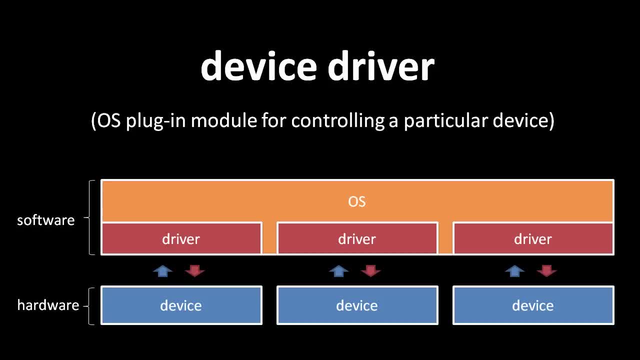 Some standardized devices may function with a generic driver. eg, a USB mouse may perform all common USB mouse functionality with a driver written for a generic USB mouse. However, many devices require a more specific driver. For example, in my system, using the generic. 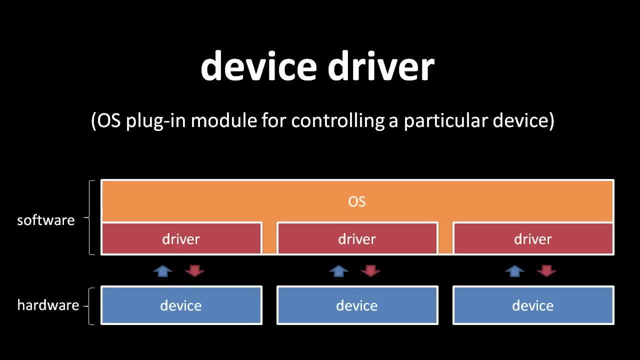 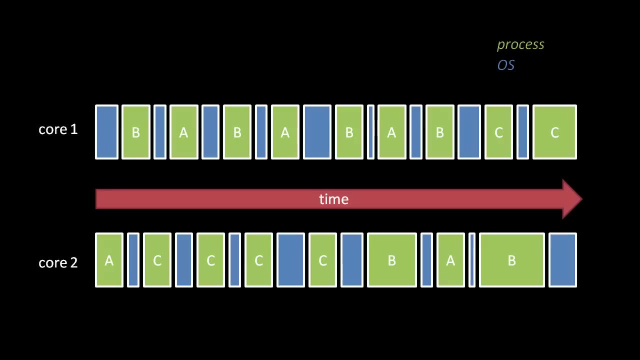 graphics driver provided by Windows only provides bare minimum functionality. To run high resolutions and play games, I must install the driver provided by AMD for my Radeon graphics card. A primary purpose of modern operating systems is to allow for multiple processes to run concurrently, meaning at the same time. The problem, of course, is that each CPU core can only execute the code of one process at a time, and the OS's own code can't run on a core at the same time as any process. The solution, then, is to have each CPU core alternate between running each open process. 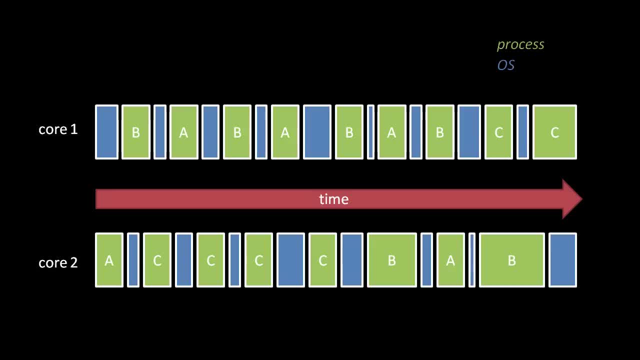 and alternate running processes with running OS code. So here, if we have two CPU cores and three open processes- A, B and C- notice that each process only runs on one core at a time. At no point does a process run on the same time. 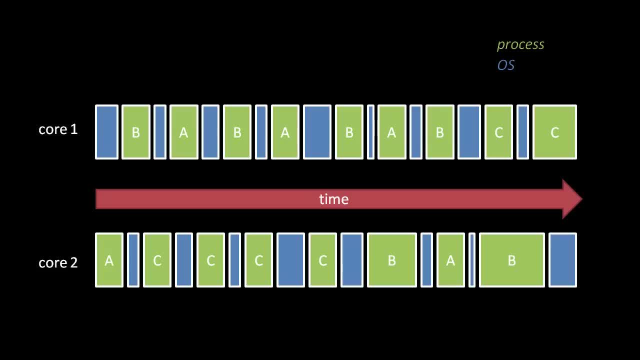 And if we counter that with a pure encoded OS, the only system that can run onto that process B run simultaneously on both of the two cores. Also, notice that OS code always runs on each core in between each process. What's happening here is that a portion of the OS called the scheduler runs after each. 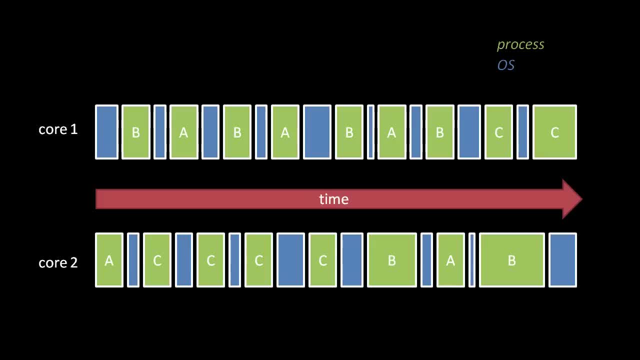 process to decide what OS work, if any should be done, and which process should run next. The question then is: how does the currently running process get interrupted? Left on its own, a running process would continue indefinitely. When any hardware interrupt is triggered, however, the interrupt handler passes off. 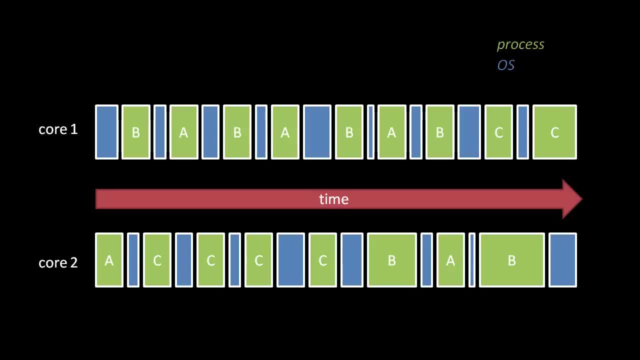 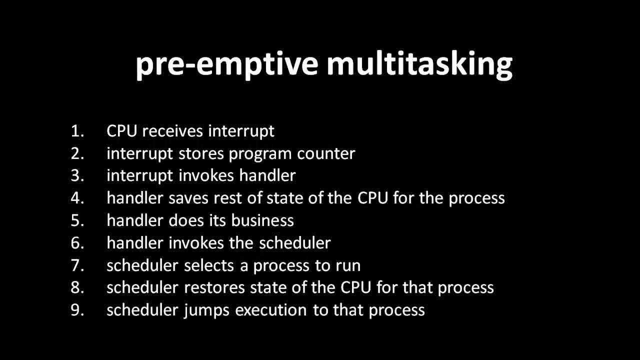 control to the scheduler, rather than handing the processor core back to the interrupted process. The scheduler then decides what OS code to run, if any, and what process should run next, Laid out in full. this scheme, called preemptive multitasking, works like this: 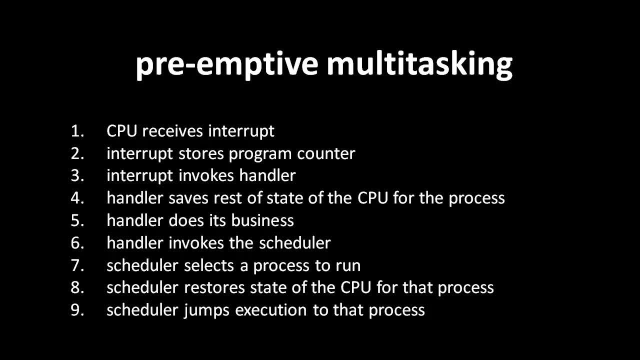 First the CPU receives some hardware interrupt. Then the interrupt stores the program counter so that the interrupted code can resume. later The interrupt invokes the appropriate handler. The handler itself saves the state of the other CPU registers so that the interrupted process can be resumed later. 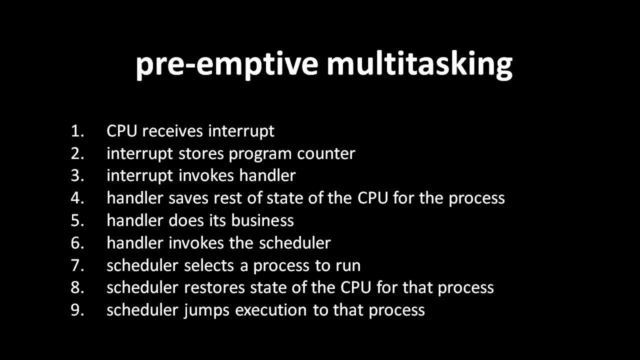 The handler does whatever business. The handler then invokes a scheduler and the scheduler selects a process to run. The scheduler then restores the CPU registers to the state they were in when that process was last running so that that process may continue. And finally the scheduler jumps execution to that process. 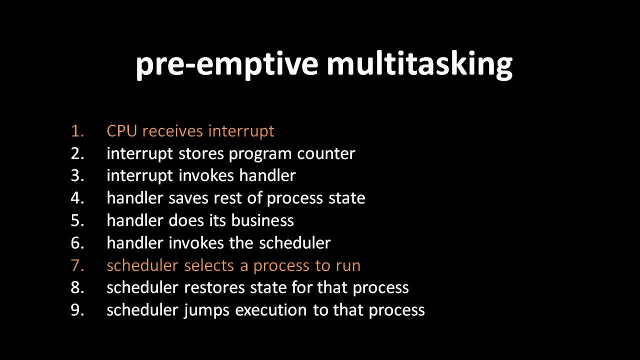 You may now be wondering two things. First, what if no interrupt is triggered by any device for a long time? That would allow the currently running process to hog the CPU, when generally we want each process to at least get a little time on a regular basis, say every several seconds or so. 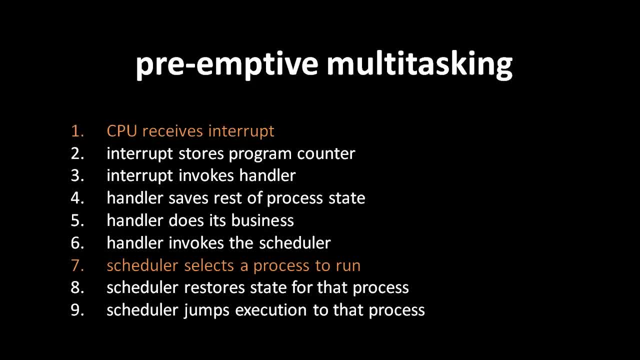 A video game, for example, typically can't go without CPU time for more than a fraction of a second, so it would be no good if some other process ran without interruption for a second or more To ensure that the scheduler gets to run on a regular basis, whether any IO devices. 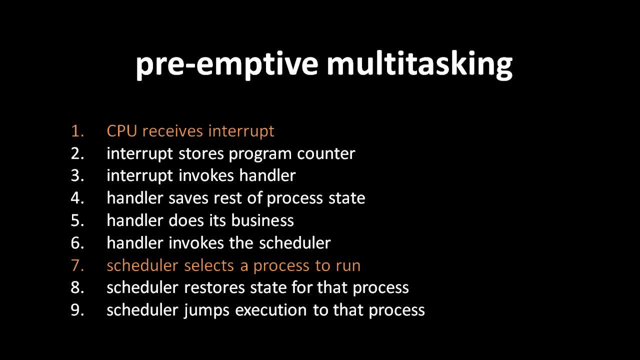 need attention or not. a clock device on the mainboard is configured to send an interrupt on a regular basis, say once every 10 or 20 milliseconds. Thus the system guarantees that the scheduler gets the opportunity to change the running process on each core at least several times a second. 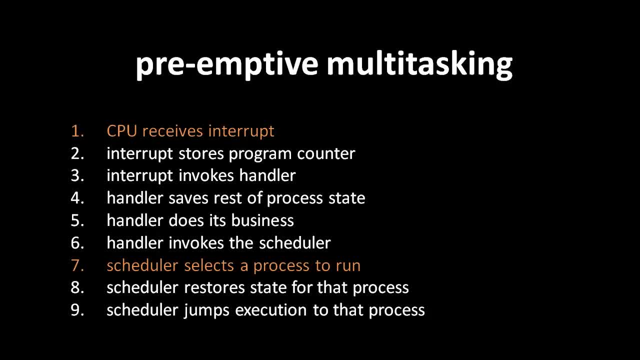 The next thing you might wonder is: how does the scheduler get to run on a regular basis? The next thing you might wonder is how the scheduler chooses which process to run next. Using the simplest algorithm, the round robin algorithm, the scheduler simply runs each. 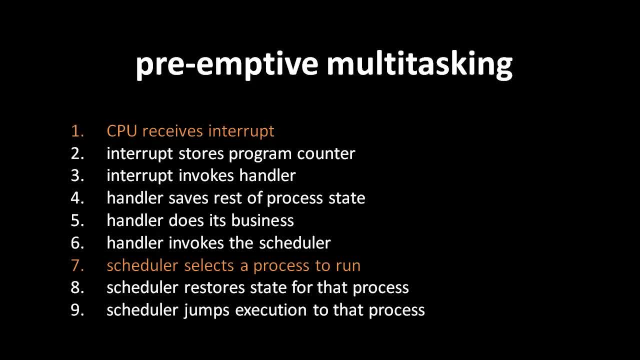 process in turn, one after the other. While this ensures that every process gets run on a regular basis, the more sophisticated algorithms used by Windows, Linux and other modern operating systems attempt to take into account which processes need processor time more than others. 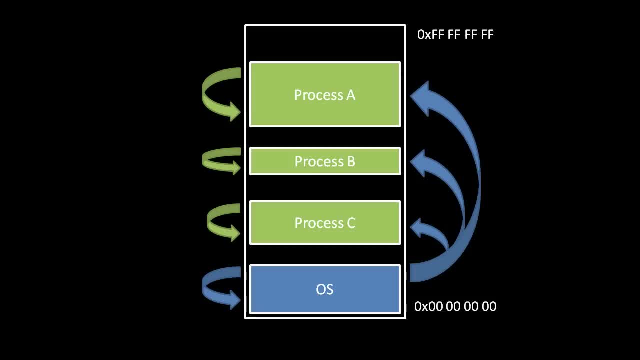 Processes not only share the CPU cores. they of course must also share the system memory. It's the OS's job to regulate the processes' use of memory, to ensure that each process doesn't interfere with the portions of memory used by other processes and by the 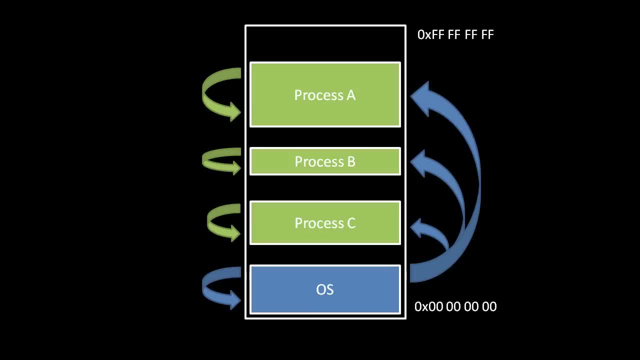 OS itself. Here, for example, the processes A, B and C have been allocated their own portions of system memory, While the OS may access any portion of memory as it chooses. because the OS is supposed to be in charge of the system, each process can only access its own portion of memory. 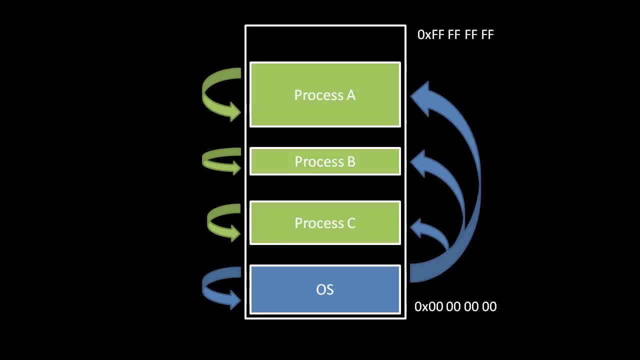 As we'll explain shortly, this restriction is enforced by the hardware, making it impossible for a process to muck with addresses. However, we need a loop hole for this restriction, because processes must be able to invoke certain routines at fixed addresses in the OS's portion of memory. 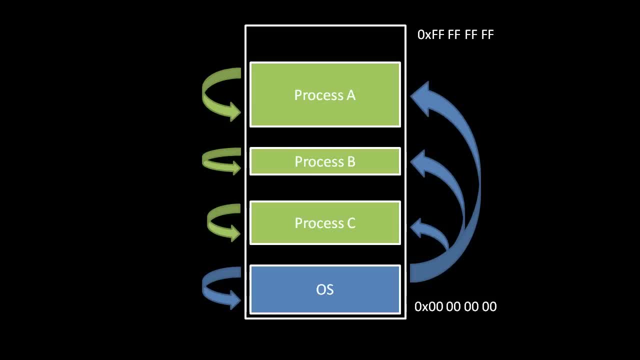 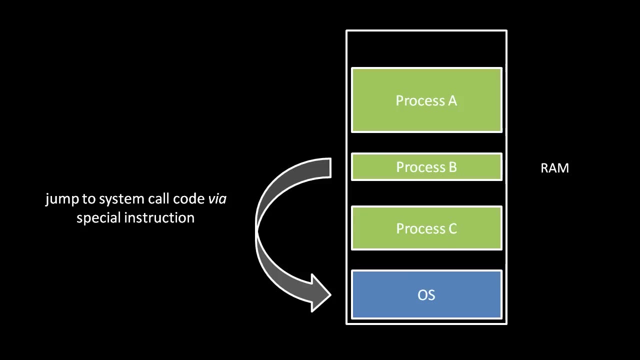 These routines, called system calls, are the means by which processes initiate requests to the operating system. These calls provide functionality for things like, say, reading and writing files, or for sending and receiving data over the network. To invoke a system call, a process must use a specific CPU instruction, usually called 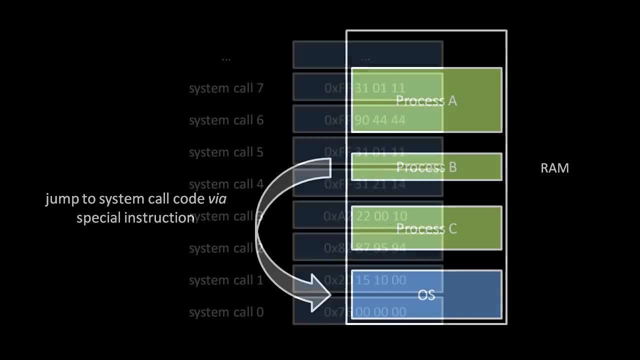 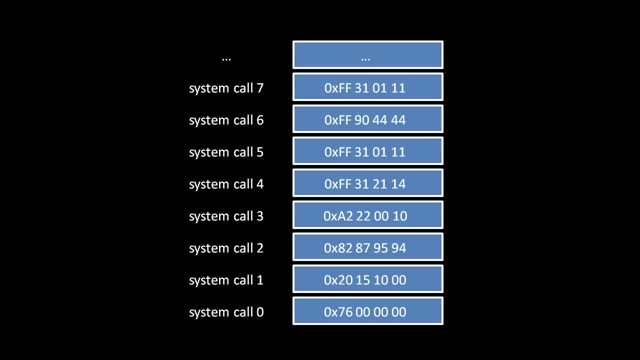 SysCall process specifies a system call number. When this instruction is invoked, the processor looks in the system call table for the address of the routine corresponding to the number and jumps execution to that address, Because the operating system controls this system call table a process. 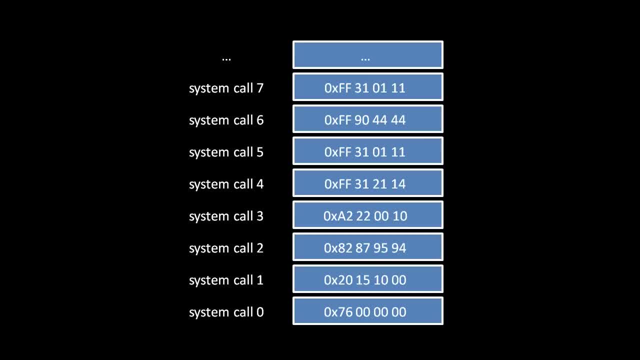 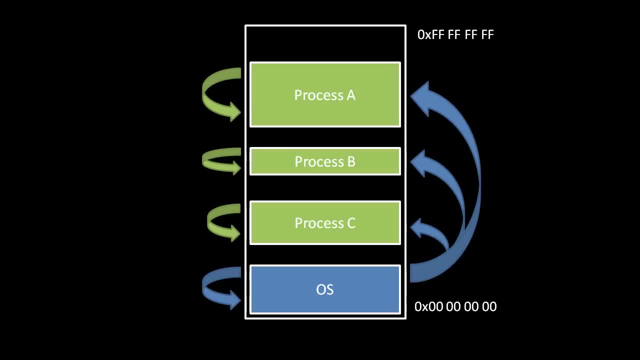 can only jump execution to addresses of the operating system's choosing. So, aside from this loophole, how do the operating system and hardware restrict a process to only access its own portion of memory? Well, first off, the CPU actually runs in two different privilege levels. When OS code 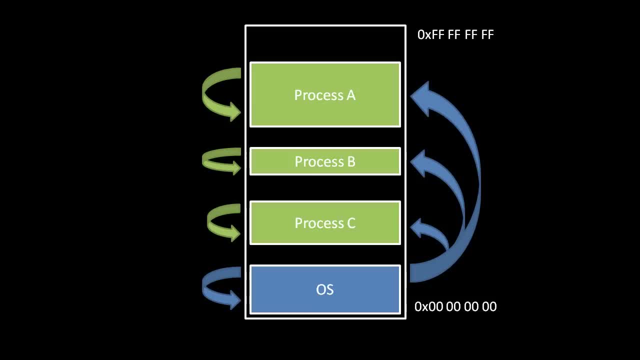 runs, the CPU is put into a privilege level that allows access of the IO devices and any address of memory. When a process runs, however, the CPU is put into a privilege level that triggers a hardware exception when the code attempts to directly access the IO devices or addresses not. 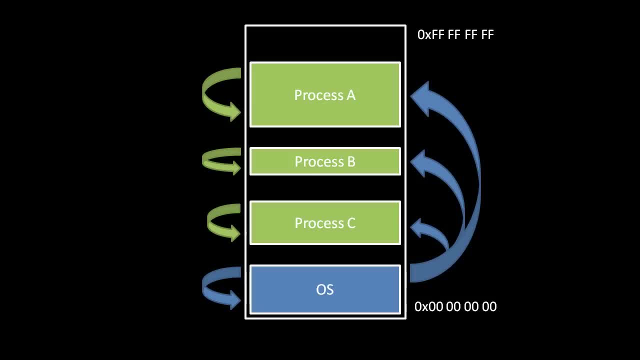 allowed for that process. Processes are supposed to directly touch only their own memory, not anything else in the system. Now, to understand how the CPU knows which addresses are allowed for each process, we have to first look at how a process uses memory. 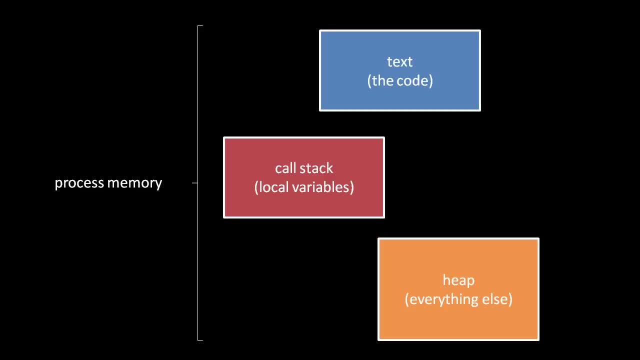 Each process uses a portion of its memory for a stack, for a heap and for storing the process's code itself in a section confusingly called the text section. even though the code is in binary form, The code section is straightforward: The binary instructions are stored in a contiguous 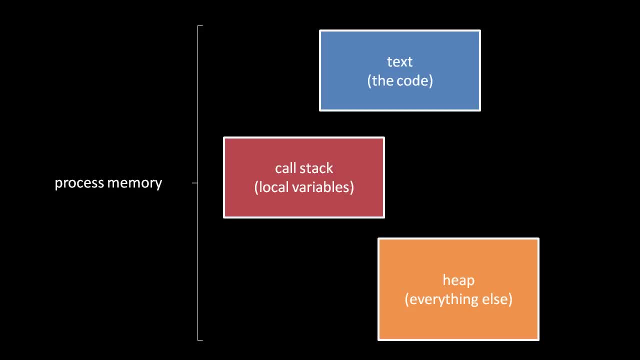 chunk of memory and never modified for the duration of the process, except for the purpose of dynamic linking with shared libraries, as we describe in the unit on programming languages. The stack and heap, though, are both for storing data. The difference is that 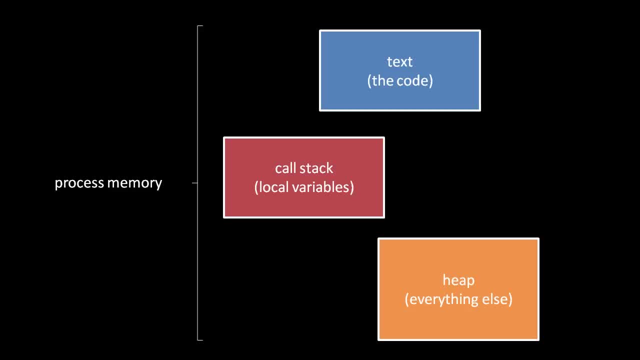 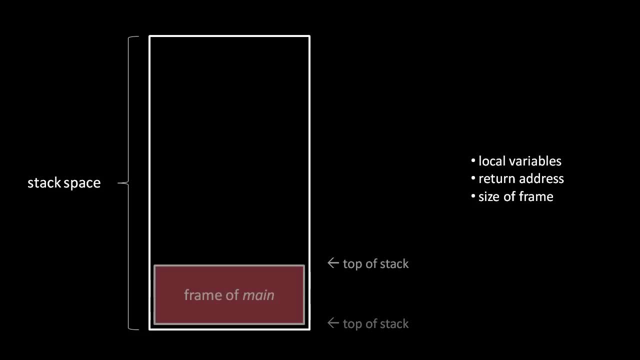 the stack stores the local variables used by the process and the heap stores everything else. Looking at the stack first. the stack is a contiguous chunk of memory that starts out unused When the first function is called. let's call it main. its local variables are stored on the stack. 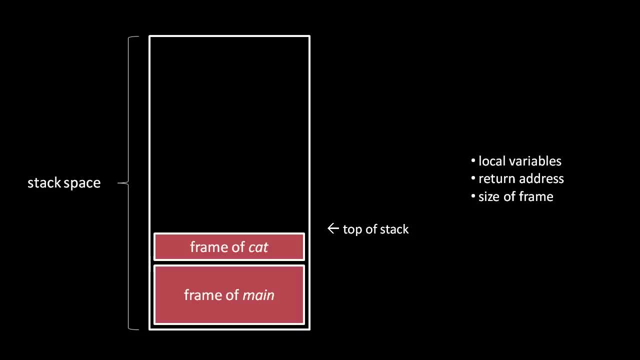 in a grouping called a frame. When the main function itself invokes another function- let's call it cat- the local variables of cat are stored in another frame on top, along with the size of the frame and the return address on the map. When the stack is stored on the main function, it looks: 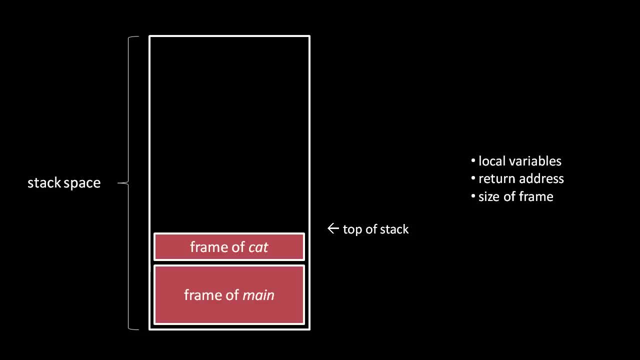 like a number with a digit, the Builder- and a tucked value on it. This number with a dot can be used to look like a number. the stack can also be marked and the stack name can be linked to the name of the return address, the address to jump back to when execution returns from cat. Likewise, if cat calls, 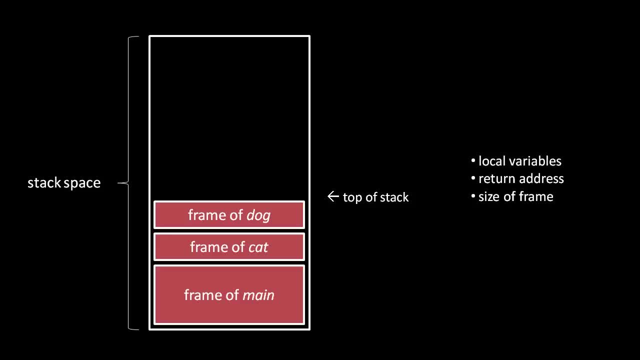 another function, dog- then dog's local variables, the size of its frame and the return address to cat are stored in another frame on top. Notice that as we add frames we have to keep track at the top of the stack, because that's where we add a frame when the next function is called. 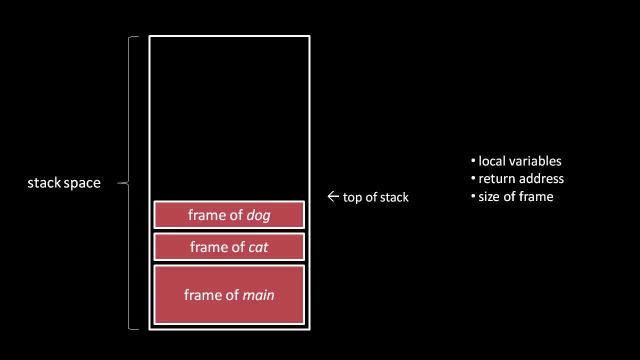 Many CPUs, including x86 CPUs, have a specific register for storing this address, usually called a stack pointer. When a function returns, the frame size is used to adjust the stack pointer back down to the last frame and execution jumps back to the return address. So when dog returns, 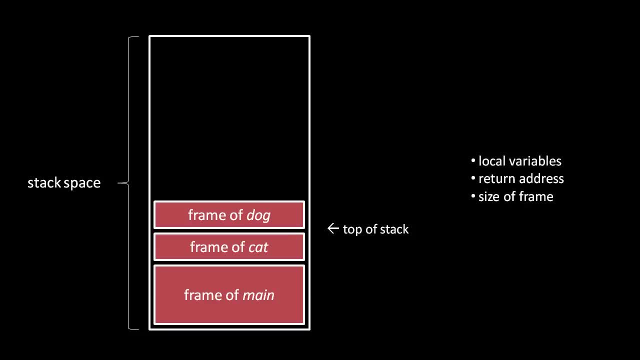 execution returns to cat and the stack pointer will point to the top of cat's frame. Notice that we don't have to actually delete any frames, because the space a frame occupies will simply get overwritten by subsequent frames as needed. Also, notice that the first frame is 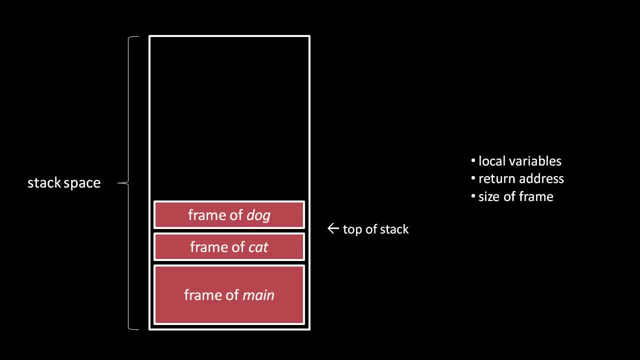 special because the program ends when the first function returns, so the first frame needs to be overwritten. So when the first function returns, the program ends when the second function returns, so the first frame needs to be overwritten. So when the first function returns, the program ends when the second function returns. so the first frame. 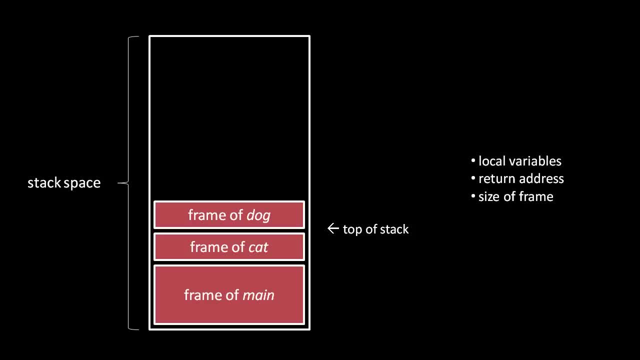 ends when the second function returns, so the first function returns Now. the diagram here suggests that the stack grows from the bottom, but in many cases the stack frames start at high memory addresses and grow downwards. This, in fact, is the case with x86 CPUs. This choice, though, is mostly arbitrary. 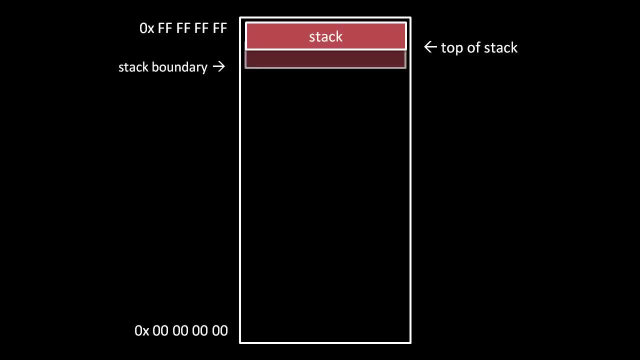 The size of the stack space in some systems is kept track of with another pointer, usually called the stack boundary, kept in another CPU register. In CPUs with this register, when the stack pointer runs past the stack boundary, this triggers a hardware exception. 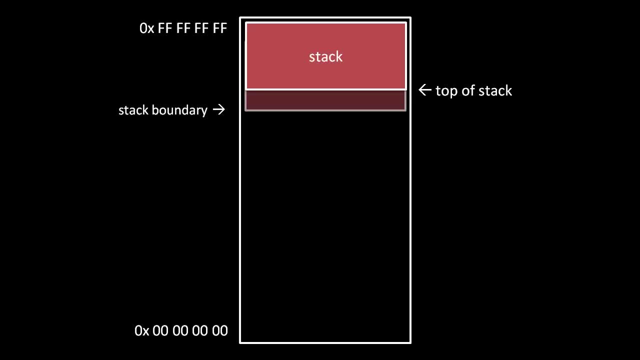 and the exception handler may increase the stack space by moving the stack boundary. However, the exception handler may decide at some point that the stack has grown too large and may simply refuse and then instead simply terminate the process. Generally, a process's stack should only get so big: a megabyte or two at the high end. 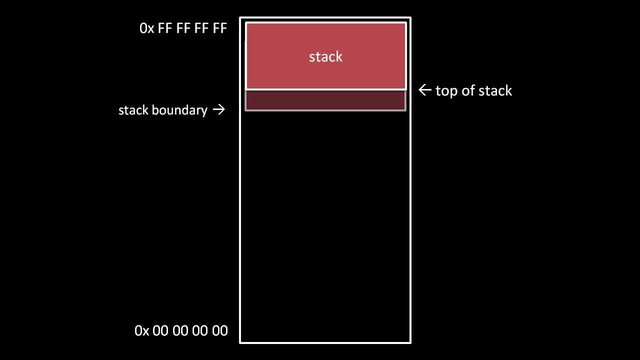 When stacks grow past this size, it's generally a sign of an underlying programming error that should be corrected, not accommodated. The most common cause of an overly large stack is an overly long chain of recursive function calls. When a program exceeds its available stack space, the error is called a stack overflow. 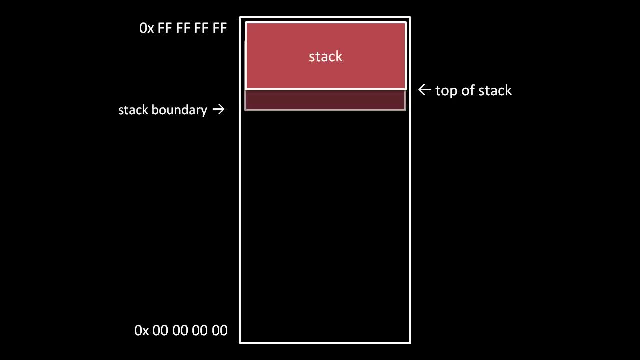 When a stack overflow occurs on a PC, the OS usually terminates the error in process. In very simple computers, however, such as in embedded systems, the stack size is not necessarily monitored with a stack boundary, and so when a program consumes more stack space than 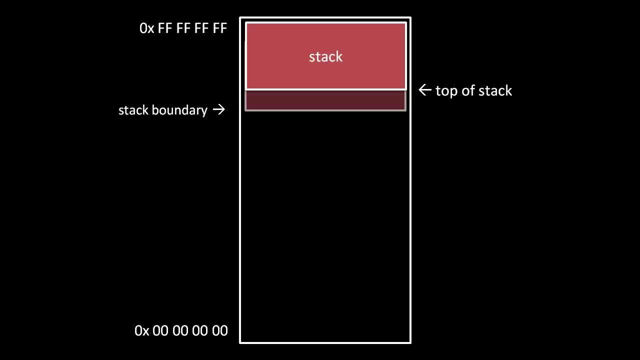 it. should, the stack may poke into parts of memory used for other data or code, likely causing unpredictable bugs. The common arrangement in PCs is to store the stack at the top of a process's address space and the text- the code- of the process- at the bottom. All the remaining space in between is 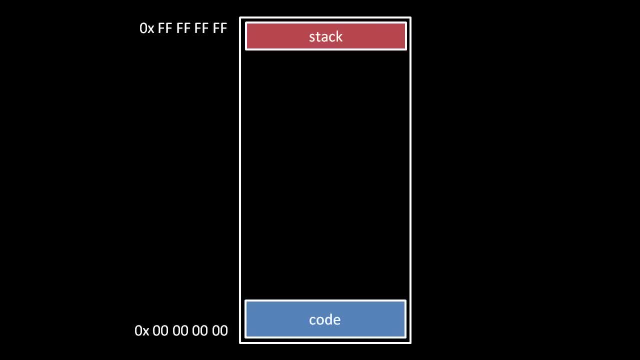 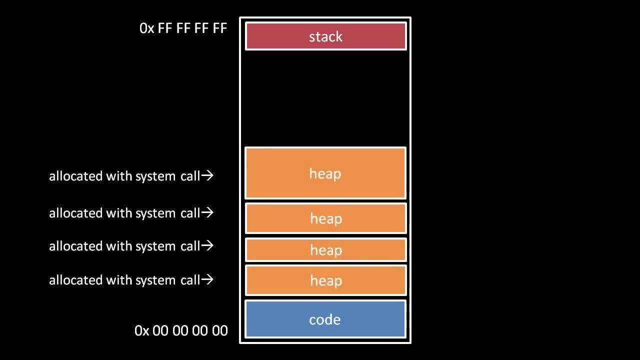 available for the heap. Unlike the stack in text, however, no heap space exists when the process starts executing. Instead, the process must explicitly request chunks of heap storage from the OS with a system call. In the call, the process specifies what size contiguous chunk it wants. 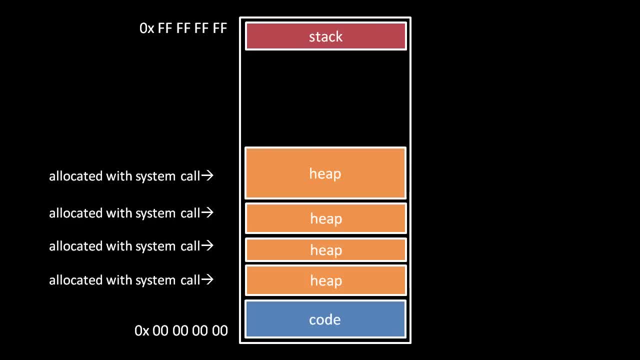 but the OS decides where to locate these chunks in the address space and the chunk locations are not necessarily adjacent. When a process is done with a chunk of heap, it should give the chunk back to the OS with a system called to deallocate. It is the responsibility of the OS to keep track of which portions of the 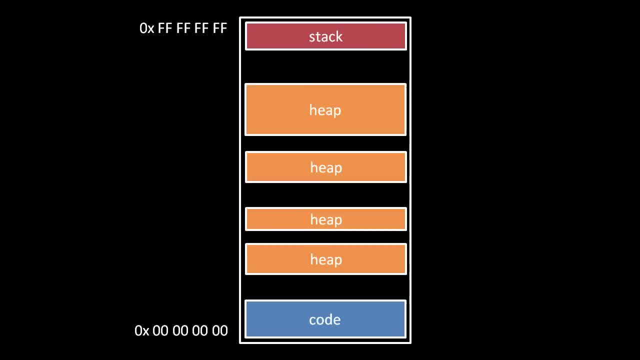 address space are free for future allocations. but notice that as a process allocates and deallocates chunks of memory, the memory space can become more and more fragmented, effectively shrinking the size of heap chunks which the OS can allocate, because each chunk must be contiguous. Here, for example, the largest heap chunk which the OS can. 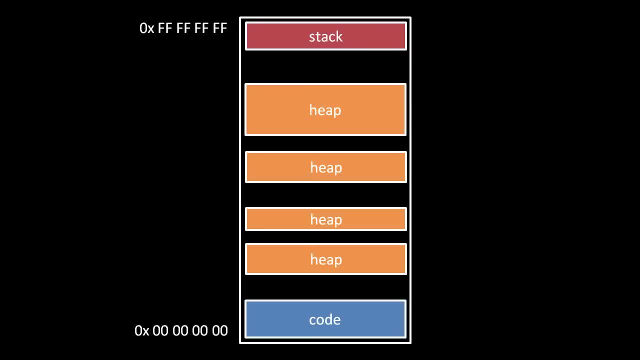 allocate is considerably smaller than the amount of free space remaining. Good allocation algorithms can minimize this fragmentation, but the problem can't be avoided entirely. This partly explains why you should deallocate chunks of heap when you no longer need them By deallocating you free up. 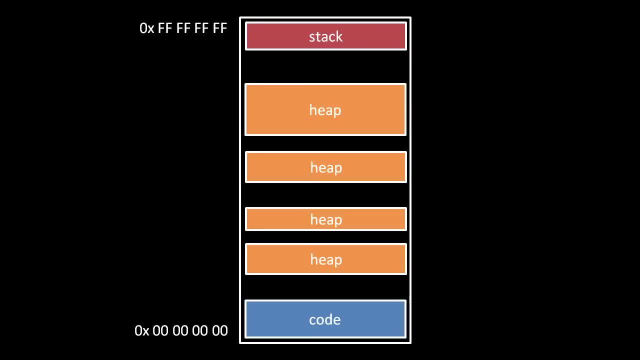 areas in the address space so that they can be allocated again later. The broader reason to deallocate, of course, is that your process might simply run out of address space at some point, Even if your process only needs a modest amount of heap memory at any one time. if your process runs, 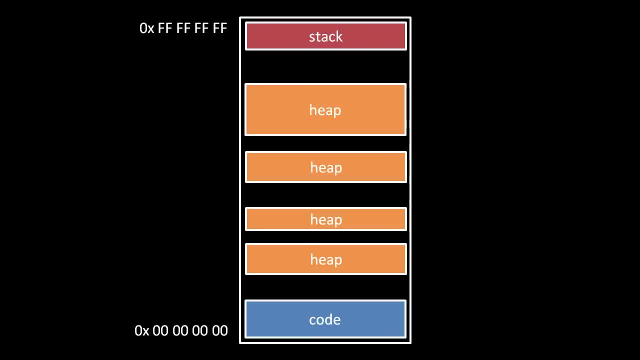 long enough, it will be able to run out of heap memory at any one time. If your process runs long enough without properly deallocating heap memory, the process may eventually run out of address space, at which point new allocations will fail, likely requiring your process to terminate prematurely. 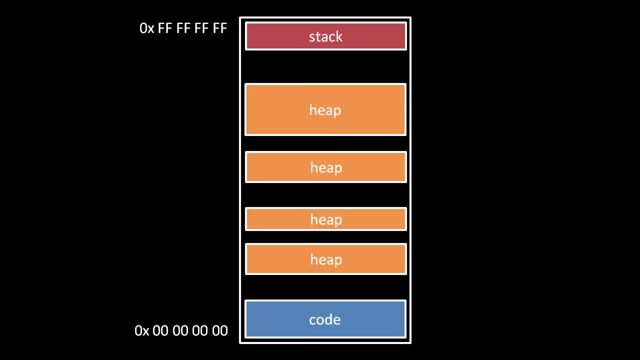 So failing to properly deallocate unneeded heap memory is generally regarded as a bug called a memory leak, because the memory available to your program effectively dwindles away over time. We'll discuss this issue in more detail in the unit on programming languages. 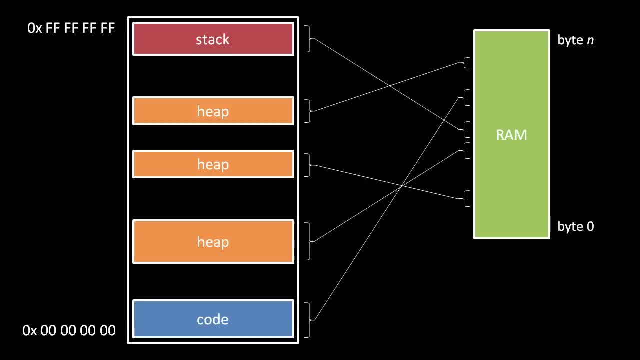 The memory addresses of a process do not actually refer to directly actual bytes of system memory. Instead, chunks of the process address space are mapped by the operating system to chunks of system memory, but not necessarily contiguously or in the same order. Here, for example, the stack is mapped to one area of RAM in the middle, the code section. 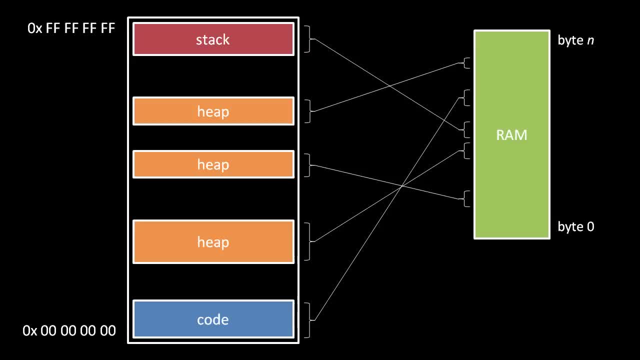 is mapped to another non-adjacent area of RAM above it, and the portions of heap are mapped to non-adjacent parts of RAM in a seemingly random order. When the OS runs a process, it lists these address mappings in a table and as the process runs, the CPU consults this table. 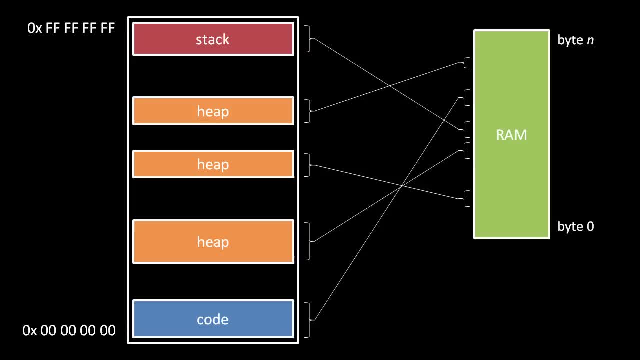 to sufficiently complete the structure of the process. For example, if the chunk of adress 0 in MotoGo is mapped to byte ffff000 of RAM, then adress 5 of the process address space translates to byte ffff0005 of RAM. 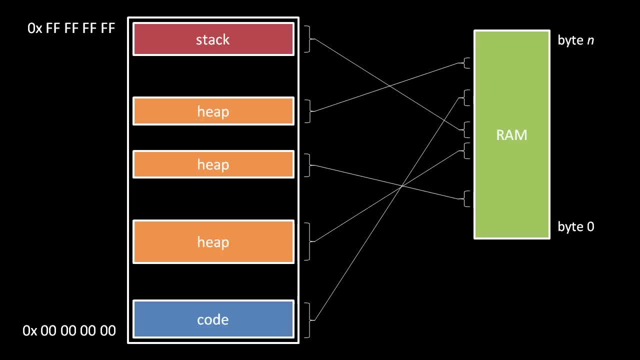 We'll also focus in a smaller building on why the opposite memory loop or process loop will Officer Run and what that doesn't achieve an duration of mission at a particular storage point of the IOM. Be clear: each processset has its own complete address space and that the OS keeps a separate. memory table for each process. Effectively, a process can be located by the OS, which is hot. This will take a couple years to extract a collection box from the process or folder while the OS is the commanding image that will have the DCMele Valleyups. 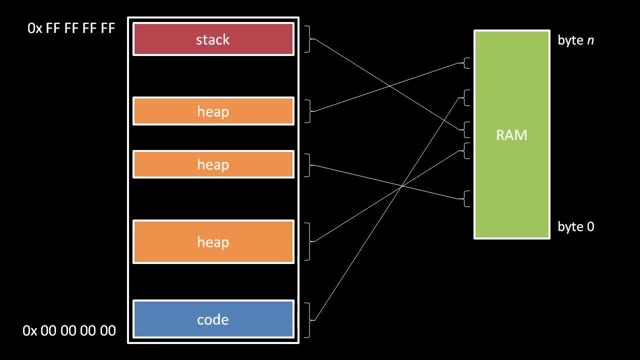 a process can be located by the OS in any part of RAM and each process can only access its own memory, not the memory of other processes or memory used by the OS. When a process attempts to use a part of its address space which is not mapped to actual RAM in the process memory table, 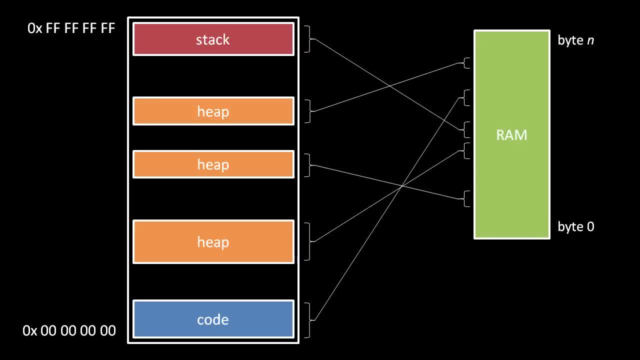 the CPU triggers a hardware exception and the OS then typically aborts the process with an error message complaining about a page fault. because the mapped chunks of memory are called pages, Each page is usually a set size which depends upon the CPU. 32-bit x86 processors. 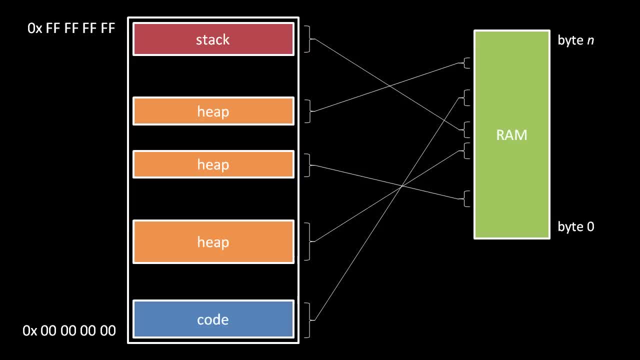 for example, usually use 4-kilobyte pages. So in fact a more realistic diagram would show that the stack, heap and code portions of a process address space are most likely not mapped as whole units, eg each page of the stack may be mapped to different, non-adjacent pages of RAM and in 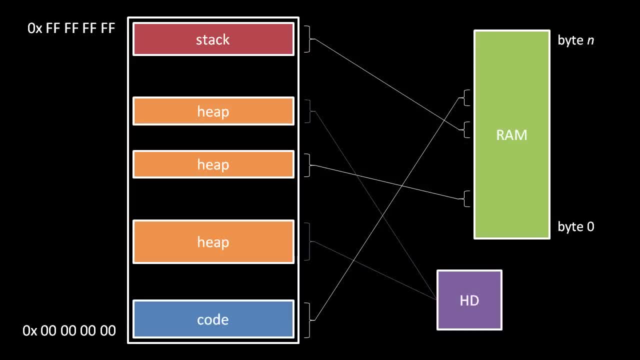 no particular order To free up valuable RAM. the OS may decide to swap out pages of a process to storage, usually a hard drive. Here, for example, these pages of heap memory are not currently mapped to any part of RAM. Instead, their data has been temporarily copied. 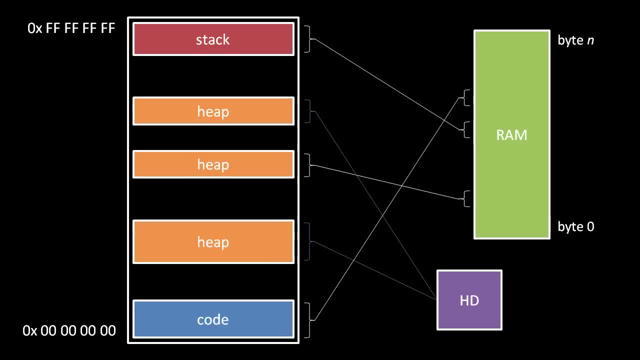 out to a hard drive and in the process memory table these heap pages have been marked swapped. An attempt by the process to access an address in a swapped page will trigger an exception, at which point the OS will copy the swapped page back to RAM and adjust the memory table. 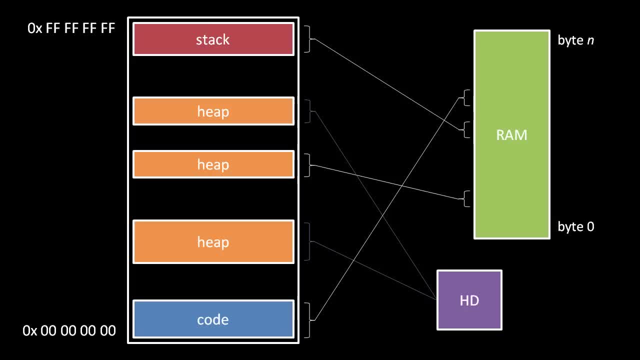 accordingly before allowing the process to proceed. Thanks to swapping, the total memory used by all processes is now a set size and the total memory used by all processes is now a total memory used by all processes. Thanks to swapping the total memory used by all processes. 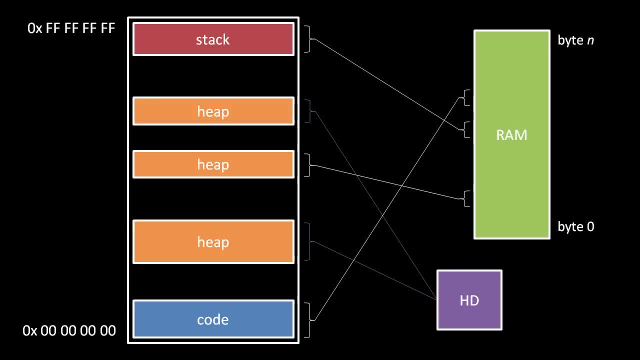 may actually exceed the capacity of RAM in the system. Swapping pages in and out of storage is of course relatively slow, but better that the system occasionally goes a bit slow to swap pages rather than simply cease to function by running out of memory. With swapping, the processes can. 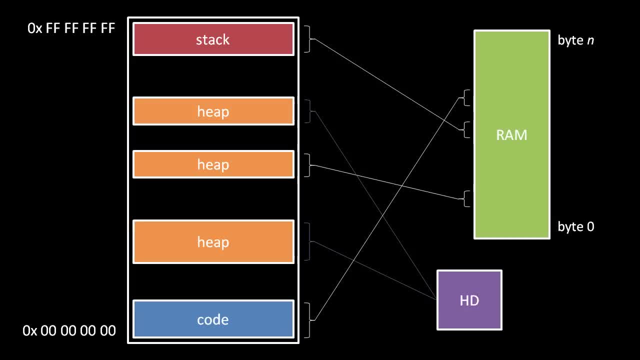 use as much memory space as a system has free storage. In practice the swapped pages in a typical PC at any moment will rarely exceed more than a gigabyte or two of storage. but most pages used by most processes don't get used very frequently, so they might as well sit in swap. 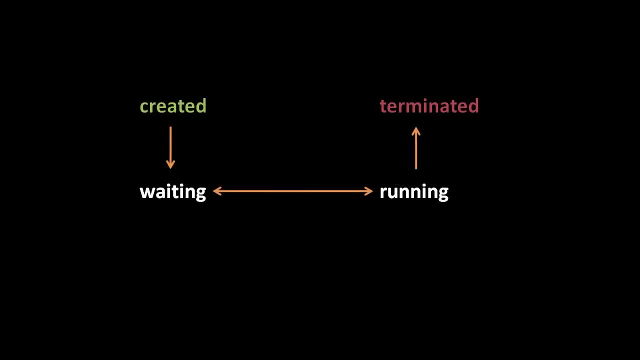 space. most of the time In its lifecycle, a process transitions through a few major states. After the OS does all the business it needs, at time of process creation, the process transitions into the waiting state. The sense of waiting here is waiting to be selected by the scheduler. When the scheduler 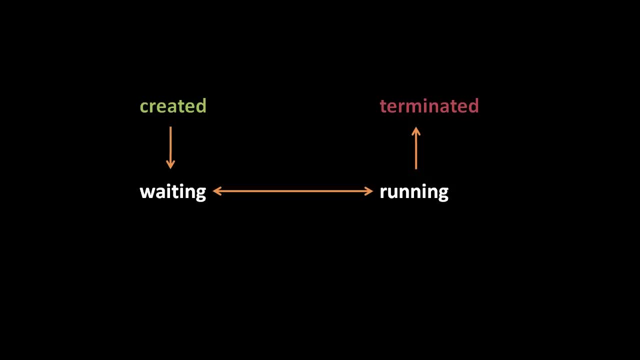 selects the process to run, it then, of course, enters the running state. When the scheduler selects a different process to run on the same core, this process is placed back into the waiting state. A process typically goes back and forth many times during the process. 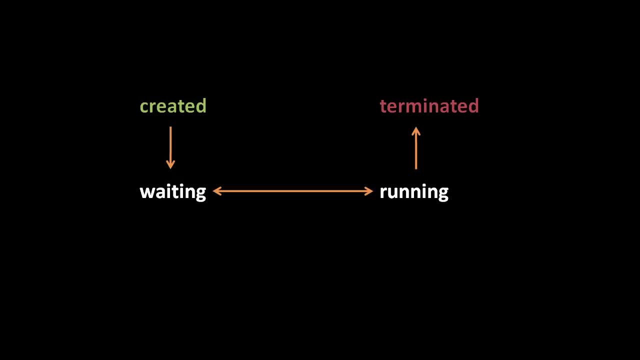 until the process ends, at which point it enters its final state terminated. There is at least one more important state blocked. In the blocked state, the process is waiting for some external event in the system before it can proceed, rather than waiting to be scheduled. so it is in neither the state of running nor so-called waiting. 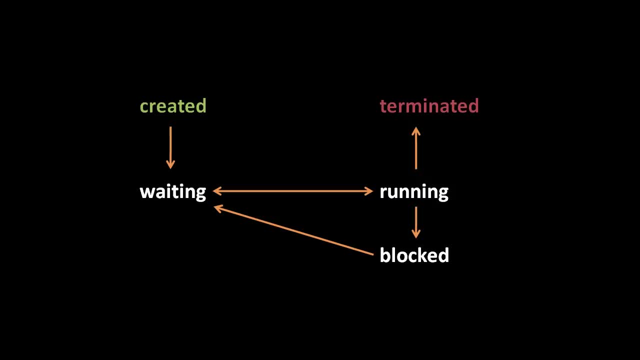 Most commonly, the blocked state is triggered when a process invokes certain system calls, such as for reading files. Reading a file often blocks a process because most stores devices, such as hard drives, are relatively much slower than the operation of the CPU, and often a program cannot do anything useful until it gets the data it needs from a file. 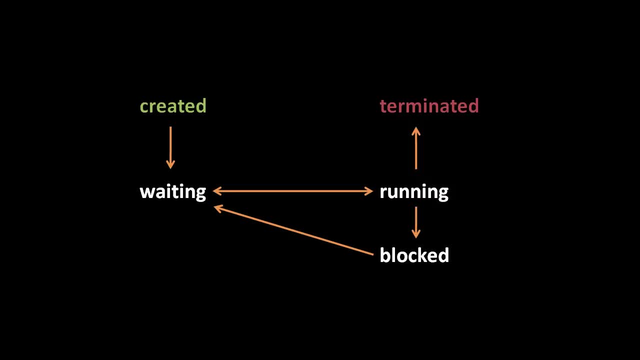 In such cases, the process might as well relinquish the CPU core it was using and take itself out of the waiting pool, allowing other processes to run while it waits. Once the operating system finishes retrieving the requested data from storage, it unblocks the process, putting 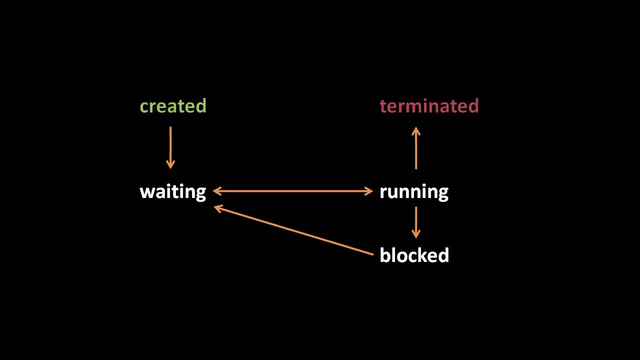 it back into the waiting state so that the scheduler will consider it again for execution. Once the operating system finishes retrieving the requested data from storage, it unblocks the process, putting it back into the waiting state so that the scheduler will consider it again for execution. 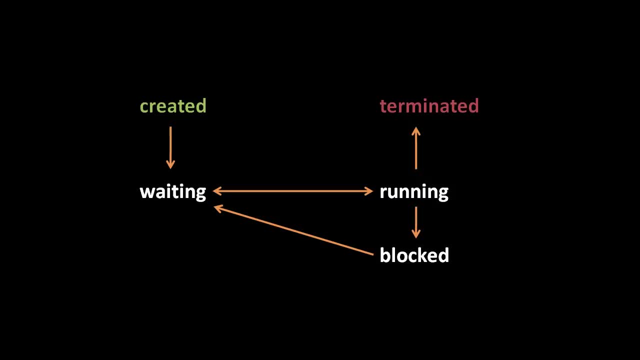 So don't get confused. Both the blocked and waiting states involve waiting, but only in the waiting state will the scheduler select the process to run. In the blocked state the process waits until the OS puts it back in the waiting state. There are several reasons to block and unblock a process, but the most common reason is because that process has to wait for some slow device in the system. 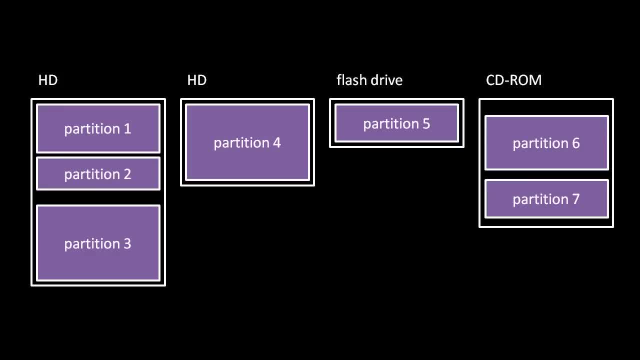 As we've mentioned, device drivers handle the business of how exactly to talk to an IO device, and that includes storage devices like hard drives. However, operating systems provide an extra layer of abstraction for storage devices, called the file system, which presents storage space as a hierarchy of directories and files stored in those directories. 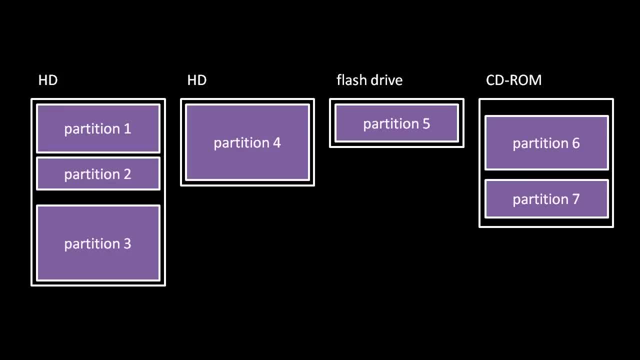 In this case, the file system is the one that is stored in the directory. The file system is the one that is stored in the directory. When your program uses a hard drive, for example, you don't want to have to concern yourself with the details of moving heads and spinning platters. 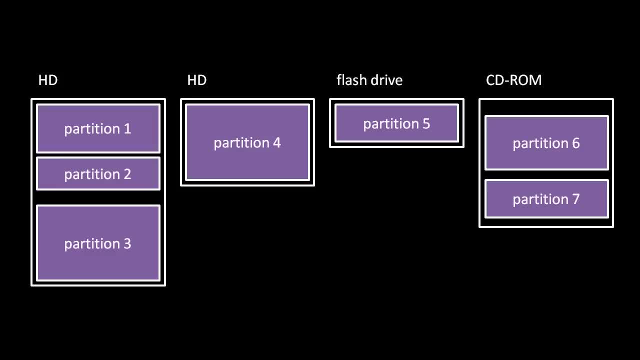 You just want to read and write data in contiguous units called files and you want to have those files organized into directories. The file system provides a subtraction allowing programmers to read and write data from any kind of storage in the same way, whether a hard drive, an optical disk, a flash drive or whatever. 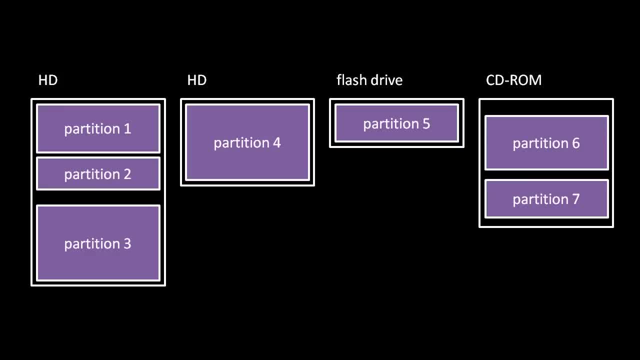 The storage area of each drive is divided into one or more contiguous chunks called partitions. Notice that some areas of a drive are divided into parts. Notice that some areas of a drive may be left blank, unformatted, such as the gap between the second and third partitions of this first hard drive. 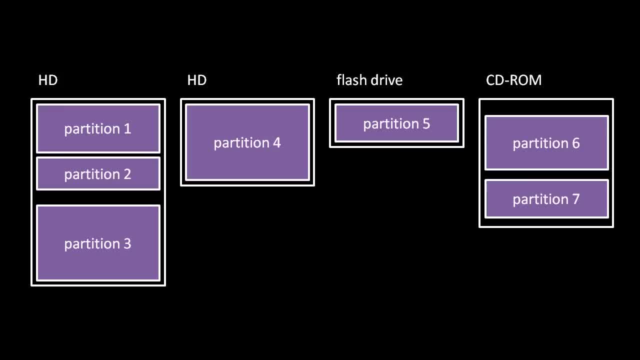 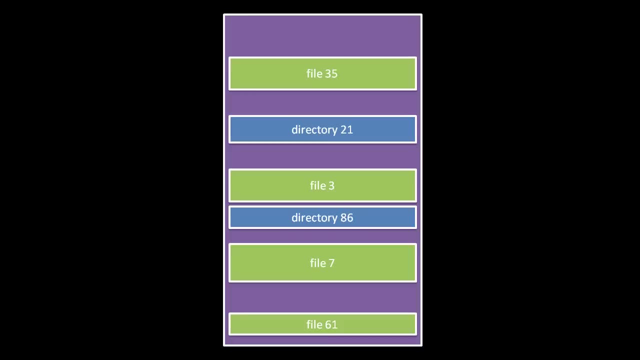 Most commonly, though, a drive is formatted to have just one partition occupying its entire storage area. Still, creating multiple partitions serves some niche use cases, such as installing multiple operating systems on a single drive. In most partition formats used today, each file and directory within a partition is known by an identifier number unique within that partition. 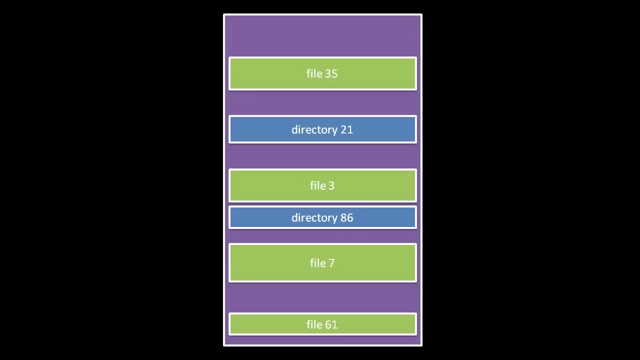 So here we have a partition with a file 35, and so we can have no other files within that partition. So here we have a partition with a file 35, and so we can have no other files within that partition with the ID 35, nor any directories with the ID 35. 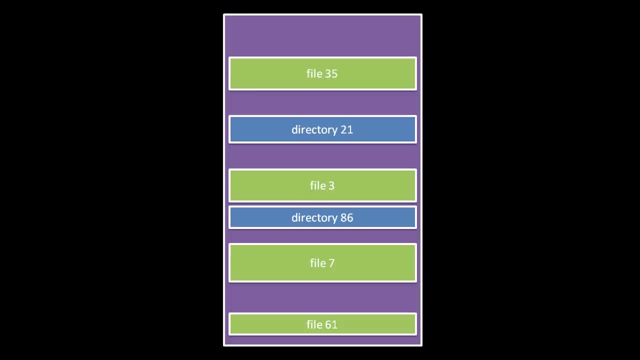 A file is simply a logically contiguous chunk of data, a sequential series of bytes. What these bytes of a file represent is entirely up to the program which writes the file. Notice, though, I said that a file is logically contiguous. When bytes are read and written by a program, the program sees them as a contiguous sequential series, but a file stored on disk may actually be stored non-contiguously and out of order. 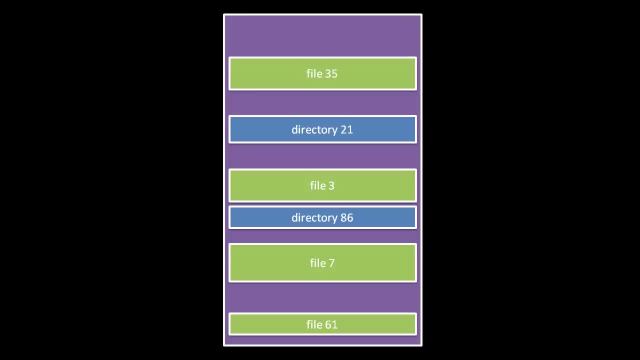 It's a responsibility of the file system to ensure that the logical order and the order of the file structure gets reconstructed when the file data is sent to a program. A directory quite simply is a list of files and other directories on the partition. 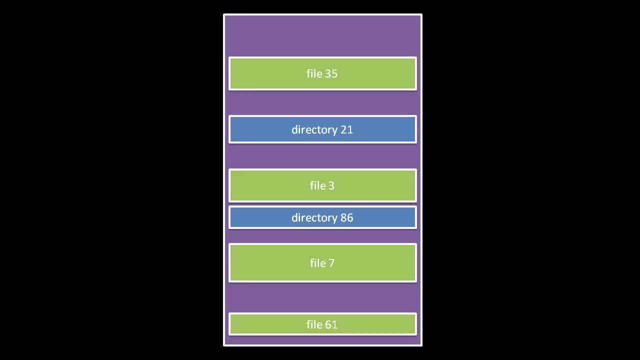 The directory associates ID numbers for files or directories with names, names which must be unique amongst all other files or directories listed in that same directory. So within a directory you can have a file and directory both named, say, Albert, but you can't have more than one file named Albert or more than one directory named Albert. 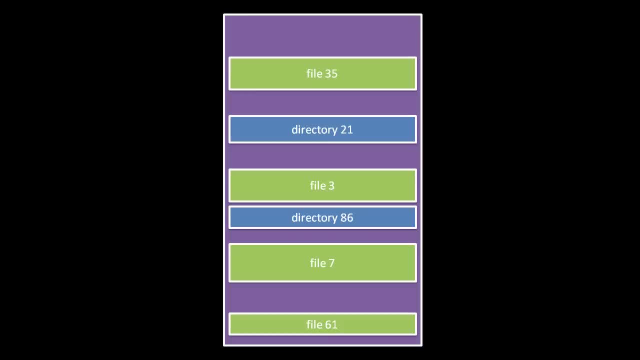 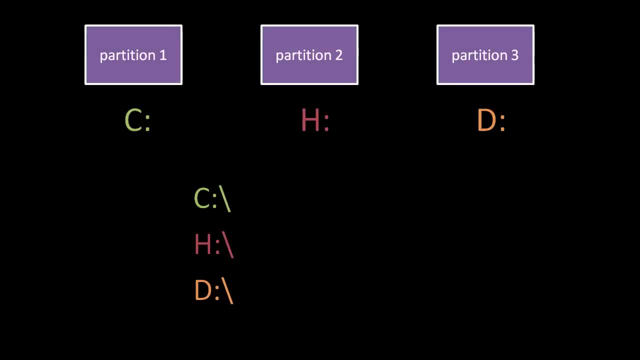 When a partition is newly created, it starts out with no files and no directories, except for one special directory called the root directory, which cannot be deleted In Windows. each partition is assigned a drive letter, usually denoted with a suffixed colon. 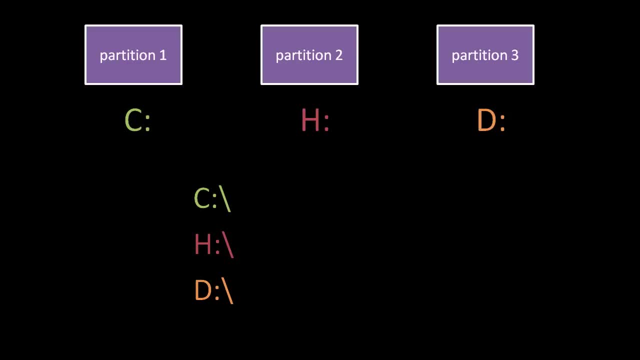 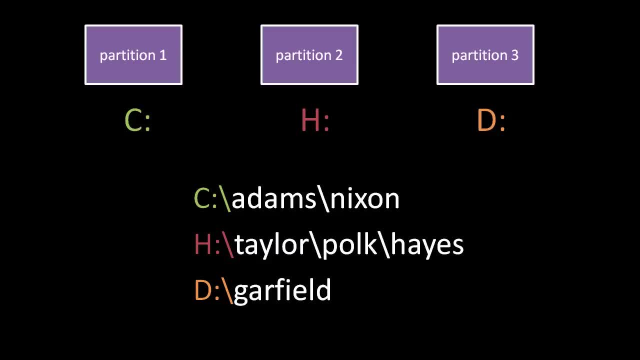 The path C, colon slash Adam slash Nixon refers to a file or directory named Nixon, itself listed in the root directory on the C partition. The path h, colon slash Taylor slash Polk slash Hayes refers to a file or directory named Hayes. 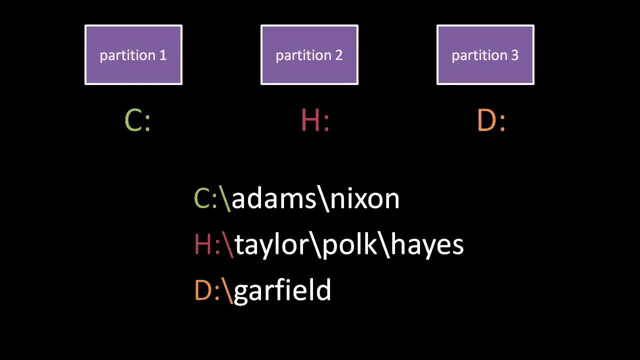 listed in a directory: Polk. listed in a directory: Taylor. listed in the root directory on the H partition. The path d colon slash Garfield refers to a file or directory named Garfield. listed in the root directory on the D partition. 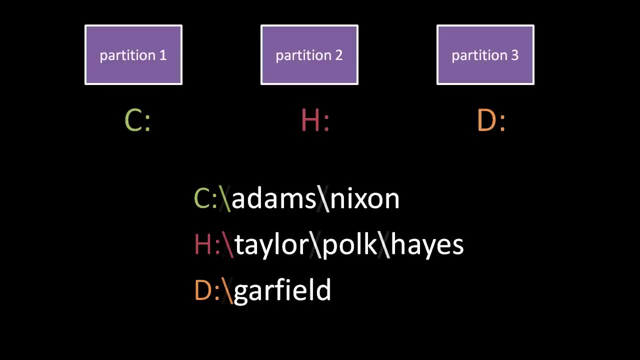 While the preferred convention in Windows file paths is to use back slashes, forward slashes work just as well. In Unix, however, file paths must use forward slashes. Ynix is blocks. major difference in Unix is that partitions are not assigned drive letters. Instead one partition. 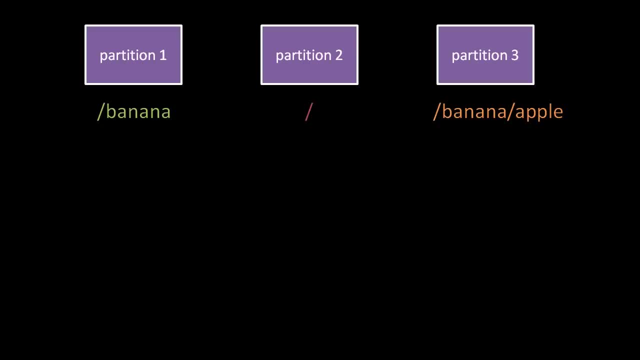 is mounted at root, meaning that the path slash refers to the root directory on that partition. Each additional partition is then made accessible by mounting it to some directory on some other already mounted partition. Here partition 2 is mounted to root and then partition 1 is mounted. 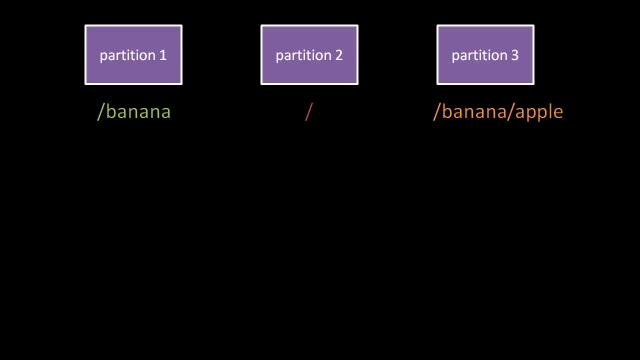 to the directory slash banana on partition 2, and in turn partition 3 is mounted to slash banana, slash apple on partition 1.. So be clear that slash banana becomes synonymous with the root directory of partition 1, such that slash banana, slash apple, must refer to a directory apple in the 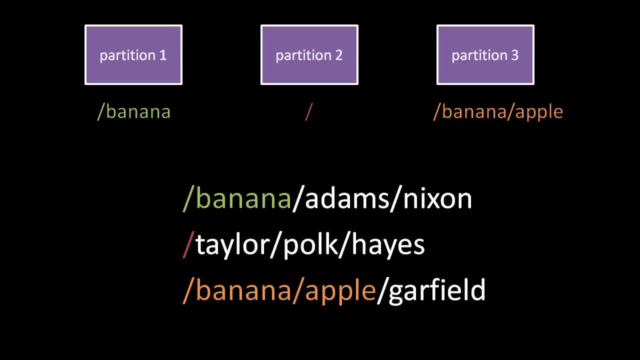 root of partition 1.. With these partitions mounted like this, the path slash banana, slash atom, slash nixon now refers to a file or directory named nixon, listed in the directory atoms listed in the root of partition 1.. The path slash taylor, slash poke, slash haze now refers to a file or directory